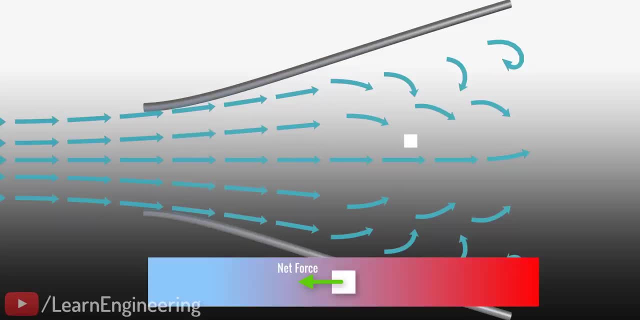 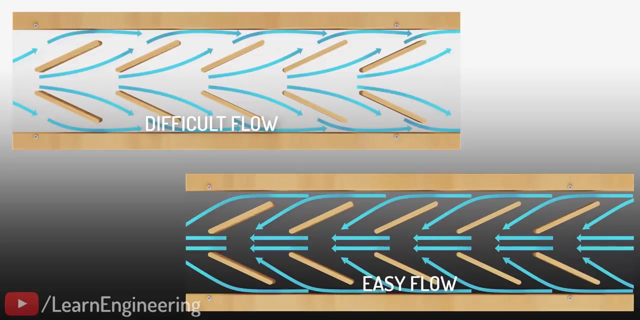 fluid particle decelerates along the length And after a particular length, flow reversal could occur. This reversal will lead to flow vortices and energy losses. In short, diverging flow is a difficult flow to maintain. It offers far more resistance than a converging flow. 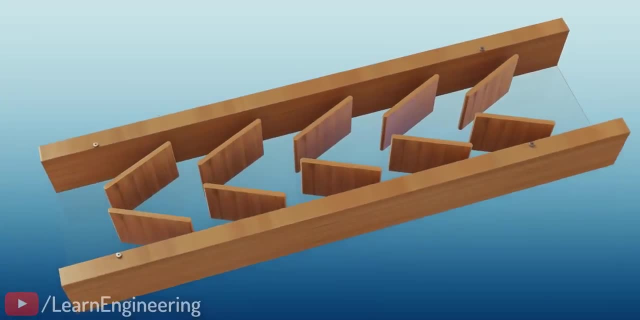 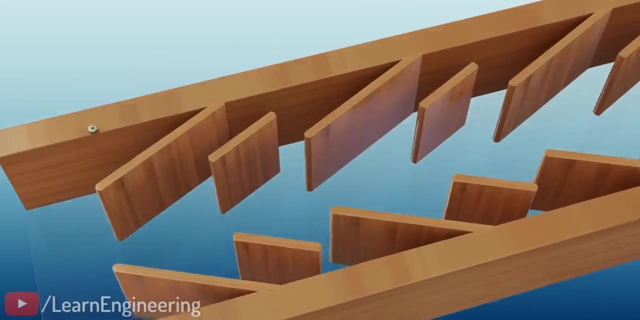 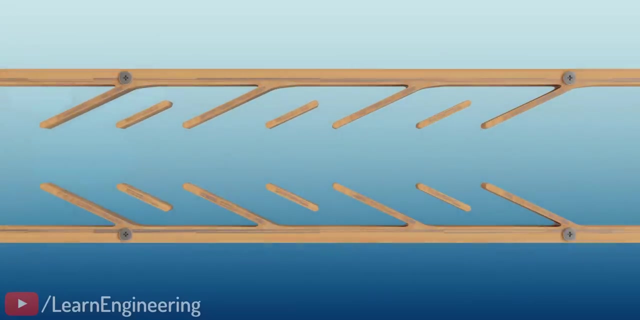 Let's rearrange the obstacles. Here, few obstacles are connected to the wall, and the ones remaining are made smaller. Let's examine what happens to the flow when it moves from left to right. You guessed it: Here the flow is getting divided into two parts, along with the flow divergence. 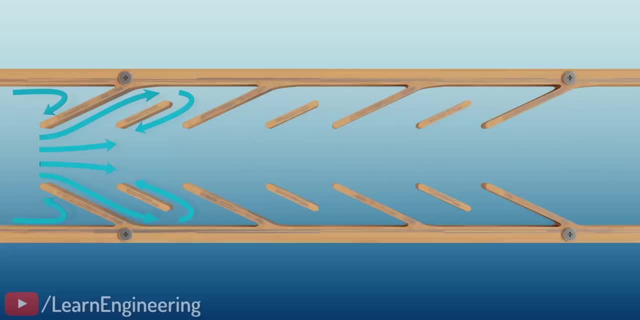 After this, the secondary streams are directed to mix with the primary stream almost in 180 degrees angle. This process is similar to mixing two jets from the opposite directions, which results in whirling of the flow and losses. This design will obviously produce more restriction than the previous design, and this process will repeat at every pair of obstacles. 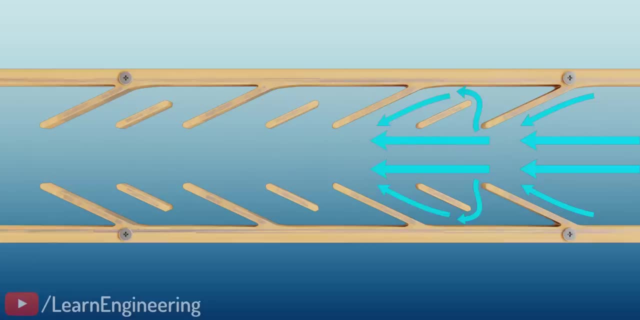 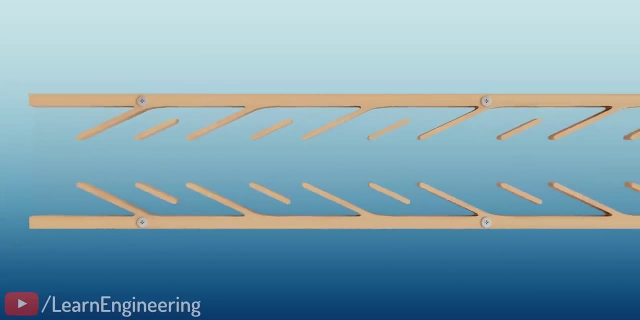 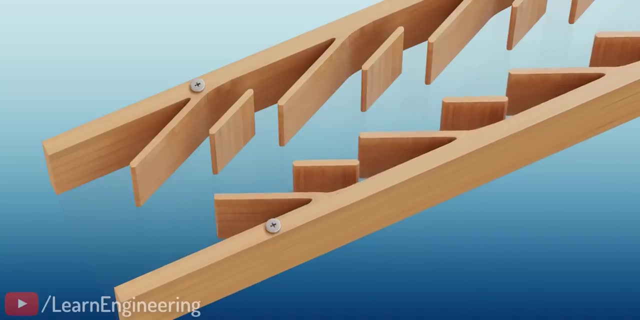 When the flow goes from right to left, it passes very easily without much obstruction. Let's make a few more geometrical modifications to this design. The previous design is a mirror reflection. Let's shift the lower portion as shown Now. the width of the obstruction is increased. What you've got now is Nikola Tesla's design. 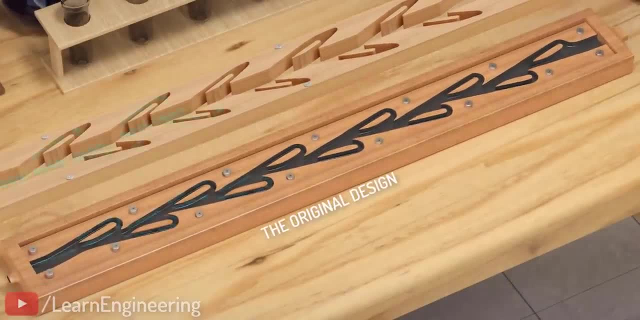 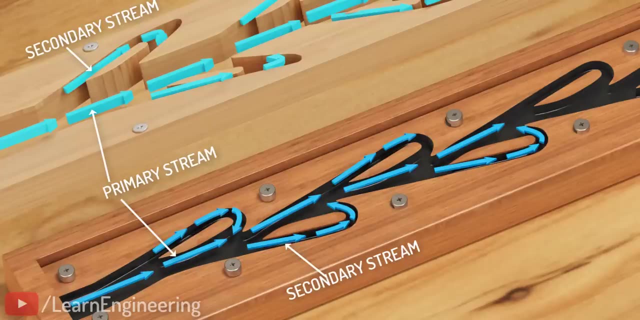 In the Tesla valve, the flow is always divided. The flow is divided into two streams: The straight-line flow is the primary stream and the diverted flow is the secondary stream. In his design, Nikola Tesla cleverly integrated all the interesting fluid mechanics we have learned so far in an optimum way. 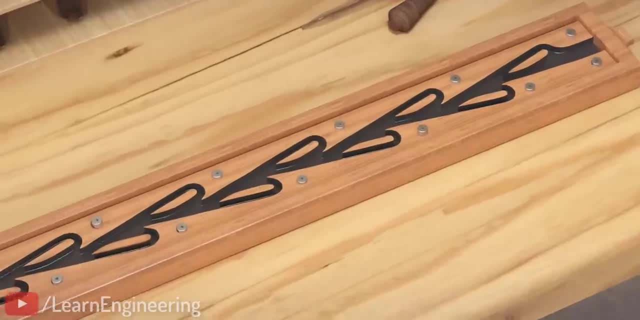 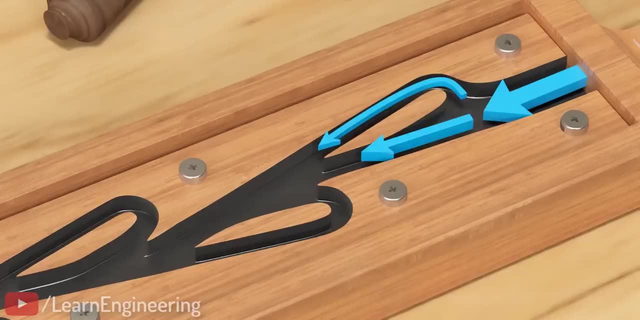 Now let's see the detailed fluid mechanics of the Tesla valve. Let's consider the right-to-left flow first. Initially, the flow is divided into two streams. Obviously, the secondary flow will be very low, since the fluid has to take an unnecessary turn to enter that region. 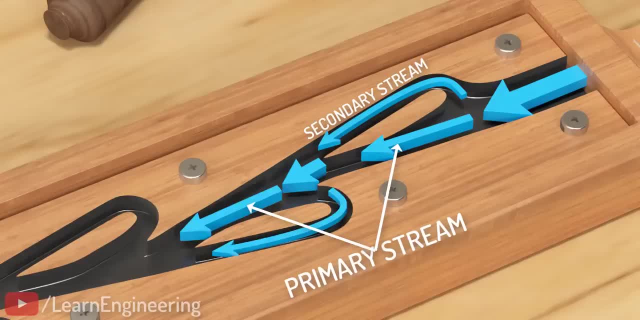 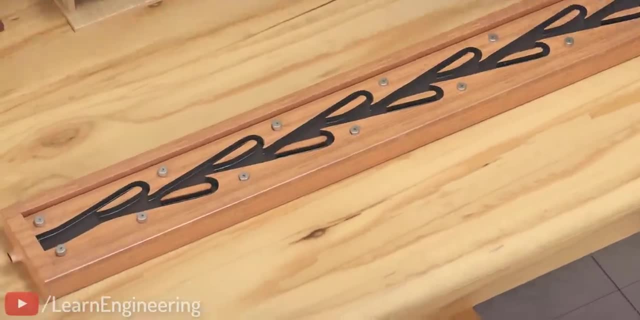 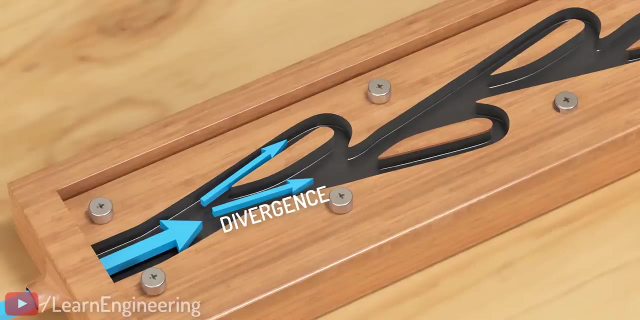 This means the majority of the flow will be due to the primary stream and it will go almost in a straight line without much obstruction. When fluid enters from the left, the flow again gets divided into two streams. In the bottom section the flow diverges and the adverse pressure gradient will make life.